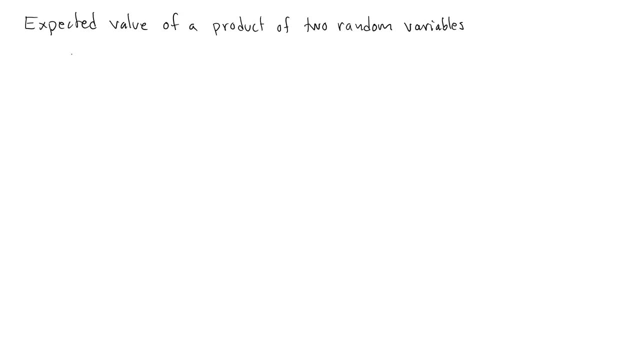 So suppose that I have two random variables, x and y. Then in general, the expected value of the product of these two random variables is not equal to the product of the expectations. x times y is a non-linear function and the expectation operator doesn't go inside. 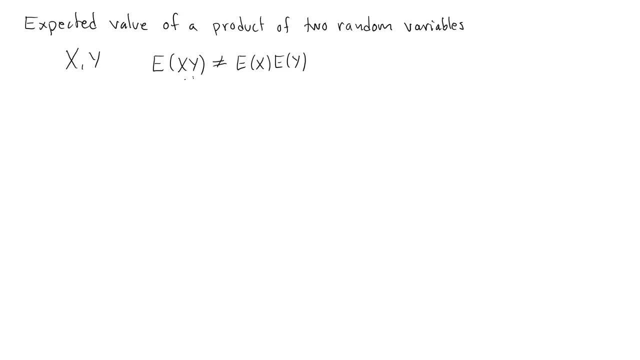 non-linear functions. It only goes inside linear functions. However, we have the following important result: If x and y are two independent, random variables, then it will actually be true that the expected value of the product is equal to the product of the expected values. It's not. 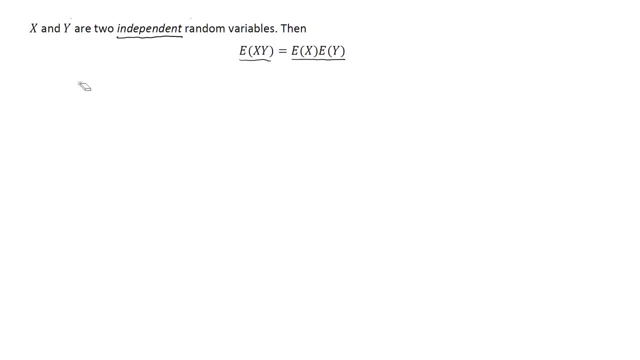 hard to show this result. if the random variables are continuous, then the expected value of the product is the 일반 consumo variable of the product. So if you look here now, this is the expectation operator конеч quicksand search term that has increased and the product of the 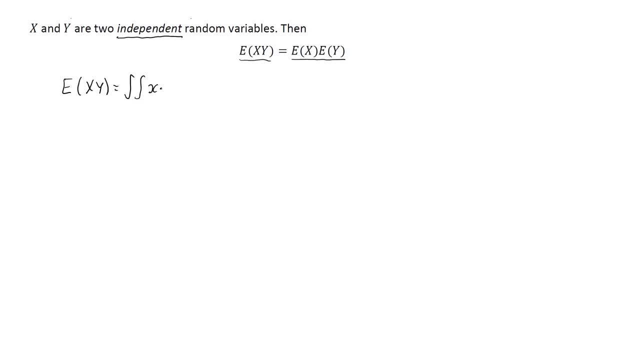 Integral of x, integral of y, x times y, f of x, y, dy, dx, where we integrate over the entire range. Well, if the random variables are independent, then the joint PDF is equal to the product of the marginal PDFs. 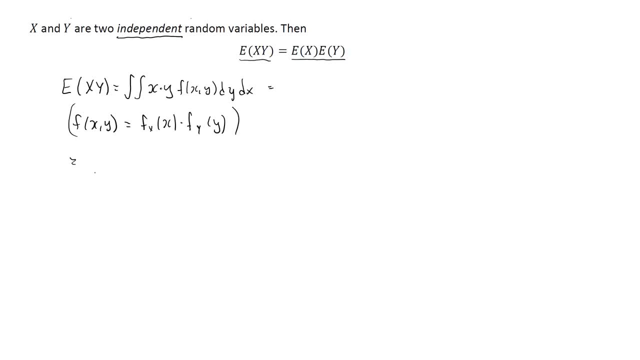 So the expected value becomes equal to integral over y, integral x times y, fx of x, fy of y, dy, dx. If the first integral is over x and the second integral is over y, we can take x fx of x outside. doesn't depend on y. 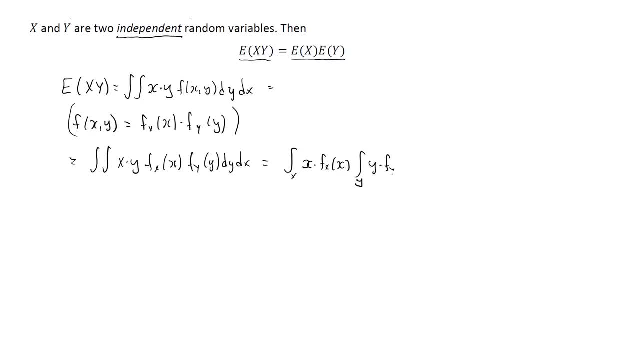 then do the integral of y, y times, fy. Okay, So we have the expected value of y, dy, then this whole thing, dx. This we recognize as the expected value of y and that now becomes a constant in the x integral.